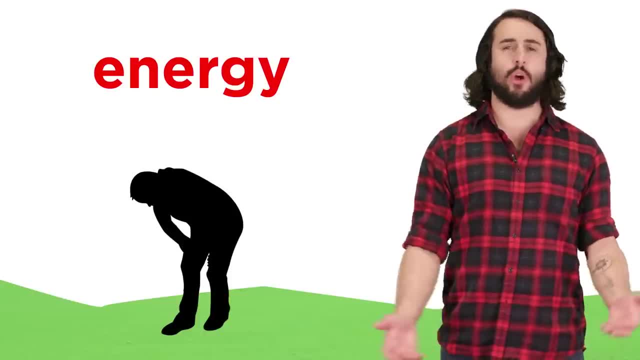 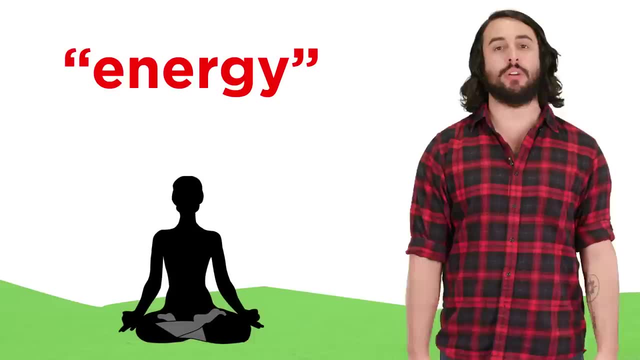 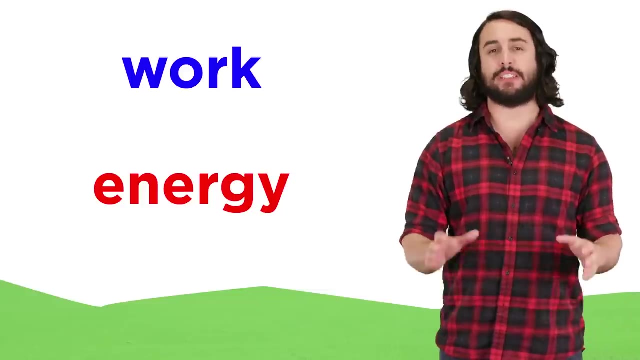 Energy is even more convoluted. We might say that today we have no energy, meaning we feel tired, Or we might use the term in a completely metaphorical way, saying that a person or a location has good energy. But once again, in physics, these words mean something very specific, and if we are to 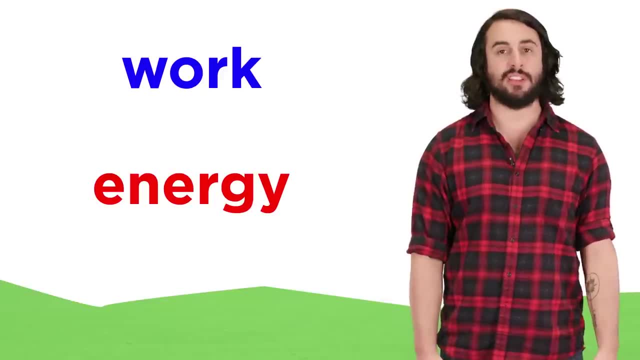 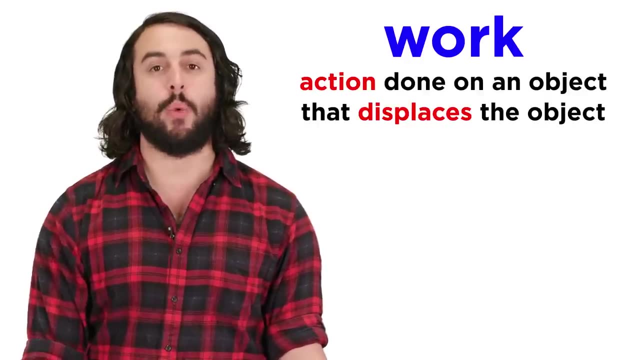 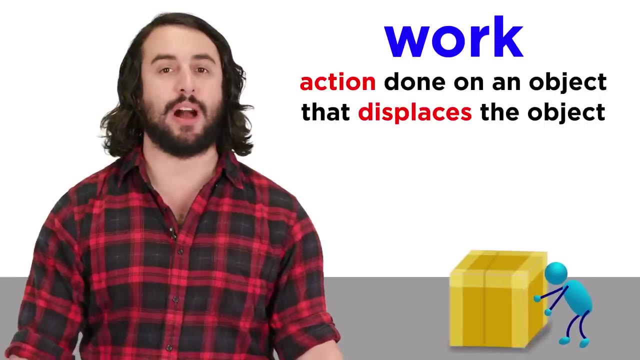 learn science. we must allow the rigorous definitions to replace the colloquial connotations. Work is defined as action done on an object whereby an applied force causes a displacement of that object. A basic example would involve pushing a box ten meters across the floor. 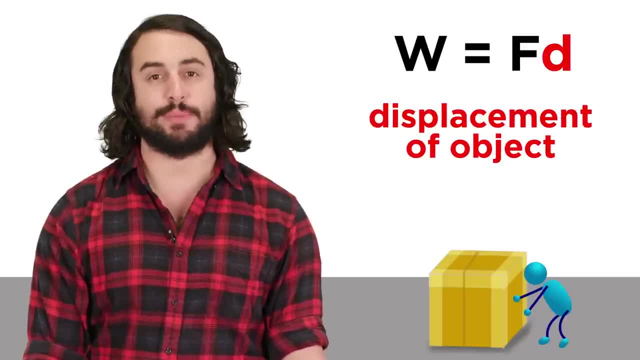 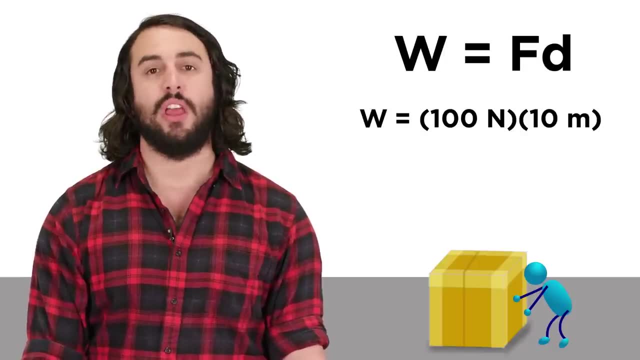 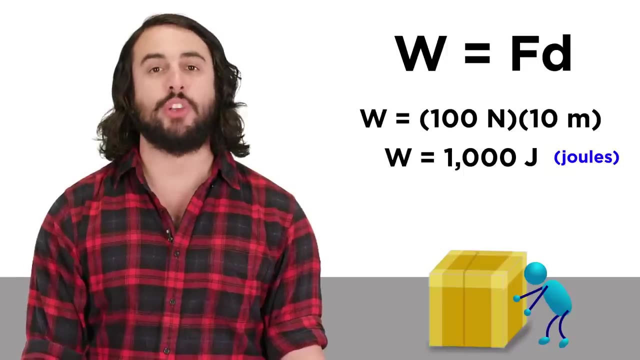 Work is equal to the magnitude of the applied force times the displacement of the object, so it has units of force times- distance. If you push with a constant force of one hundred newtons over the ten meter distance, you would do one thousand newton meters of work which are equivalent to another SI unit called joules. 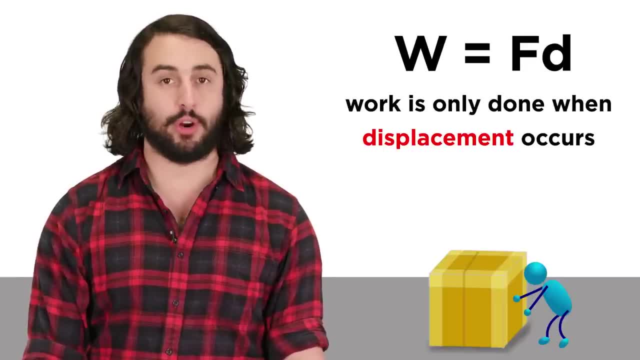 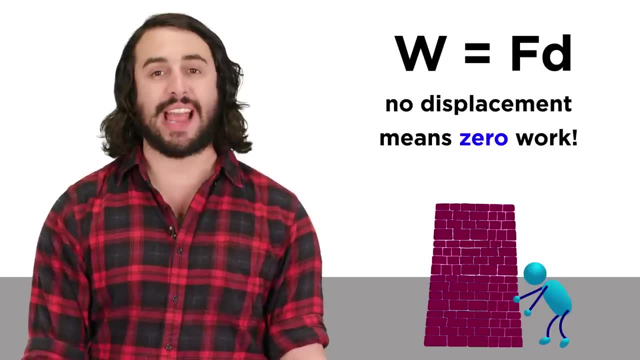 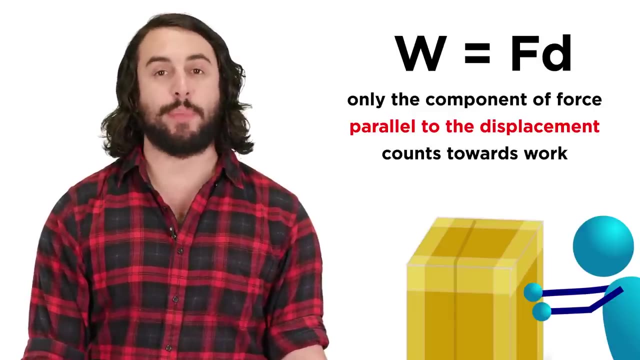 This means that work can only be done when displacement occurs. If you push a brick wall with the same force for the same amount of time as the box, you may get very tired, but technically you have done zero work. In addition, only the components of the applied force that are parallel to the displacement. 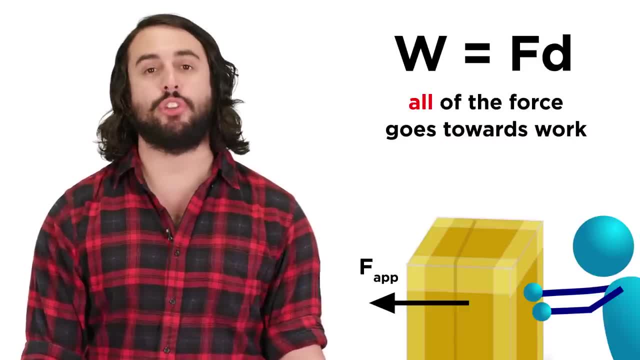 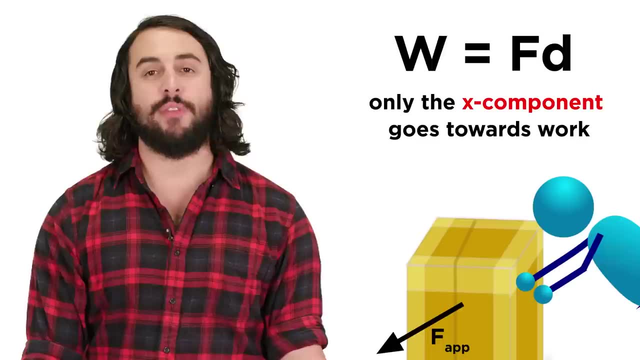 are considered to be contributing to work. If you push the box with your arms parallel to the floor, all of your effort contributes to work done on the box. But if you push the box with your arms parallel to the floor, all of your effort contributes to work done on the box. 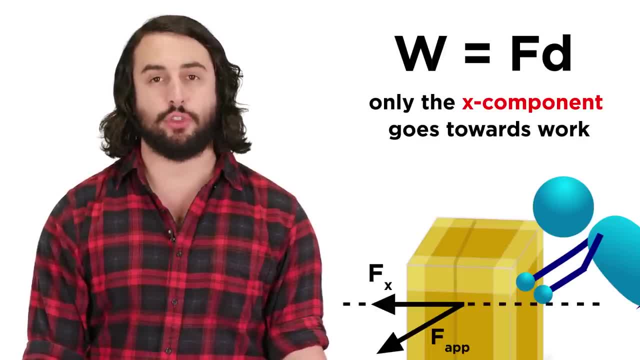 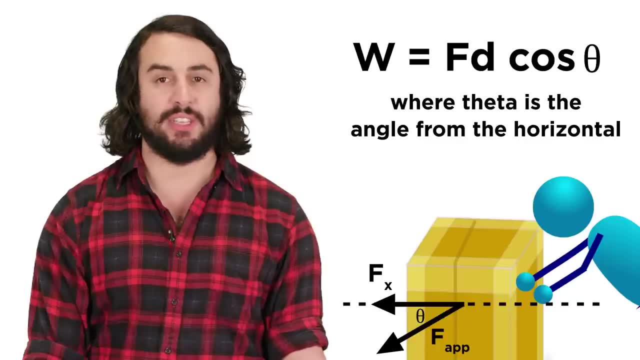 If you are pushing at a downward angle, only the x component contributes to work, while the y component does not. In such a scenario, instead of using w equals fd, we could calculate the work done on the box using w equals fd, cosine theta, as this will give us the portion of the applied force. 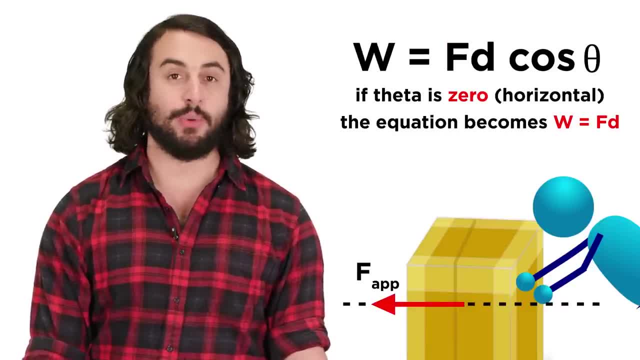 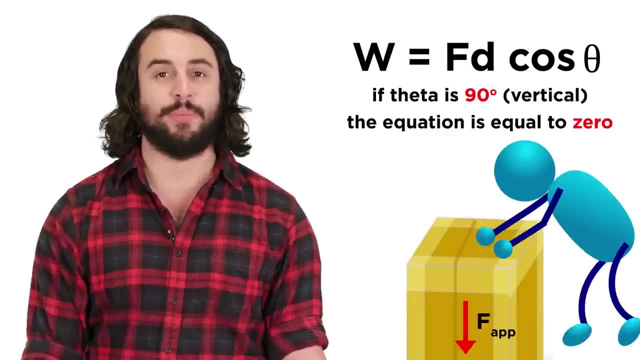 that is operating in the horizontal direction. If theta is zero, meaning the applied force is horizontal, cosine theta will be equal to one, leaving us with w equals fd, and if you were to push straight down on the box, theta will be 90 and cosine theta will. 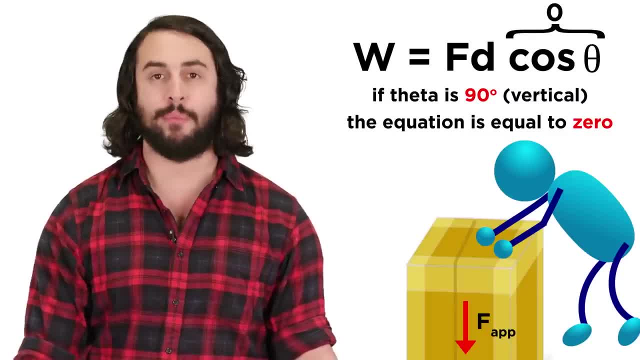 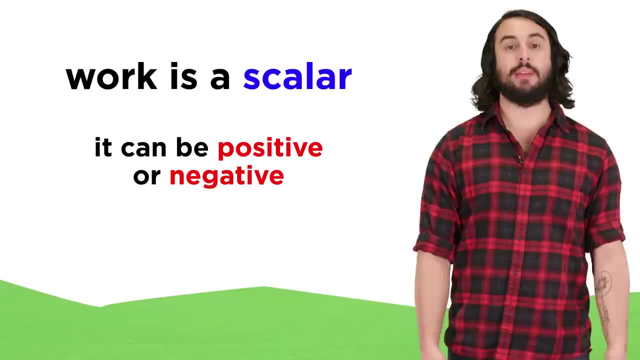 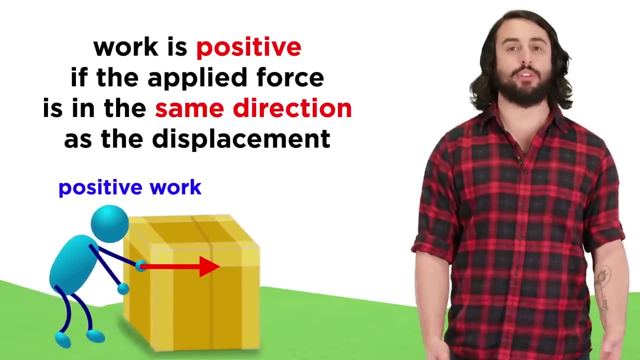 be zero, meaning no work is done on the box, and it will not move Any angle in between, and there will be some motion. We must bear in mind that work is a scalar and it can be positive or negative. Work will have a positive value when the applied force is in the same direction as the object's. 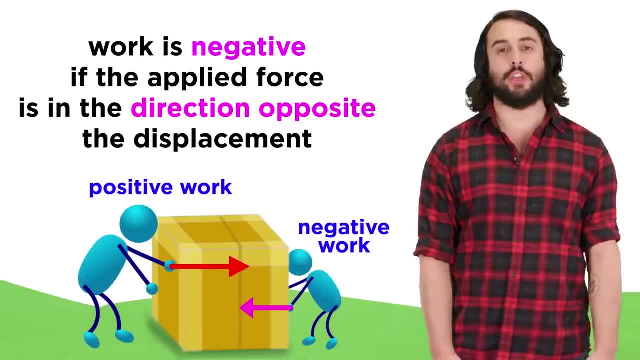 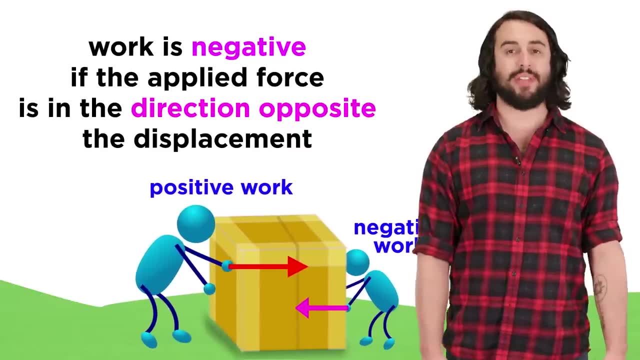 motion, like when pushing the box and work, will have a negative value if the applied force is in the direction opposite the object's motion, like if your baby brother pushes the box the other way, but without enough force to stop it from moving forward. 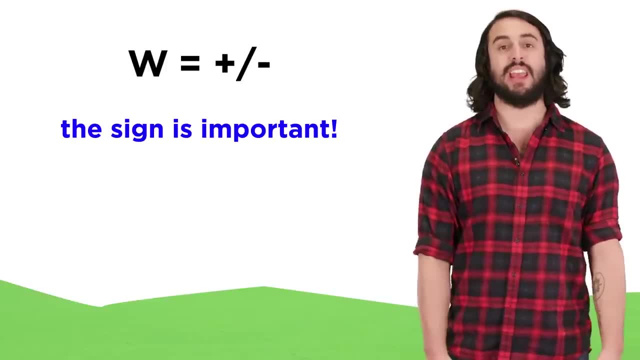 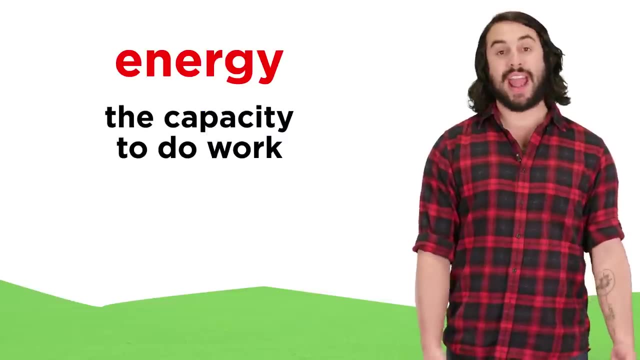 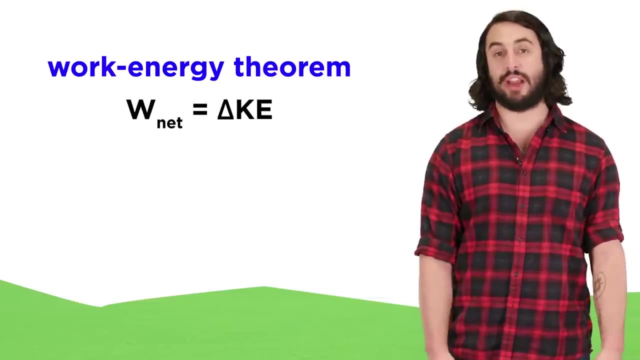 The sign on work is very important because it tells us if the speed of an object will increase or decrease as a result of applying the work Energy. another elusive term is quite simply the capacity to do work, and this is summarized in the work-energy theorem. 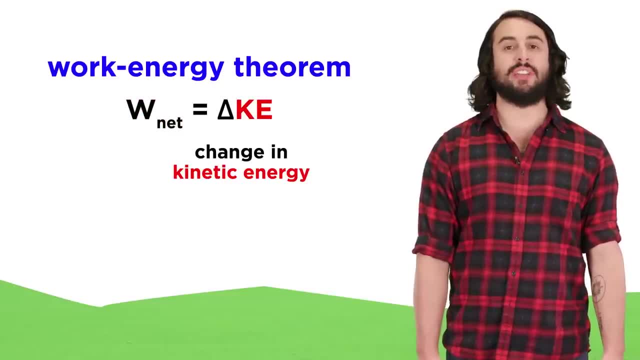 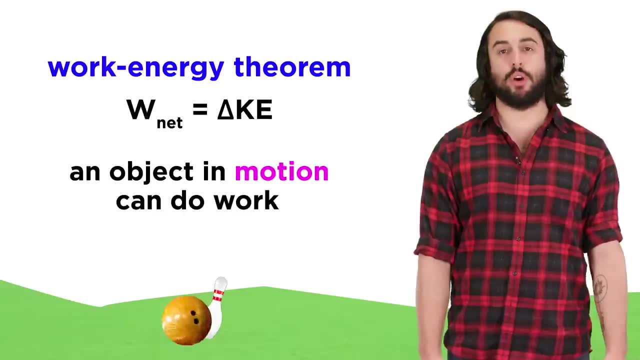 This states that when work is done on the box, theta will be 90 and cosine theta will be zero. When work is done on an object, there will be a change in that object's kinetic energy, which is the energy of motion. This also means that an object in motion is able to do work on another object. 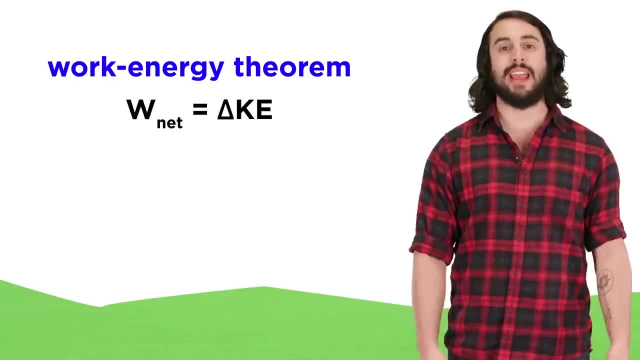 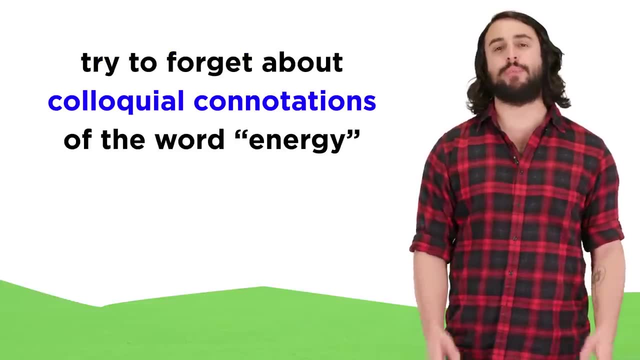 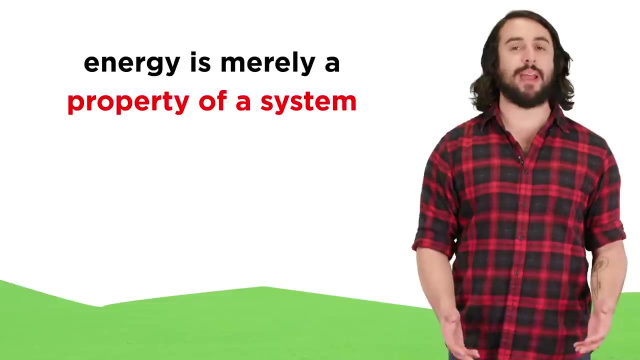 The work-energy theorem brings together concepts from Newton's laws and kinematics to describe motion in a way that we will examine further in the next clip. For now, we must simply purge ourselves of any prior connotations of the word energy and understand that it merely describes a property of a motion. 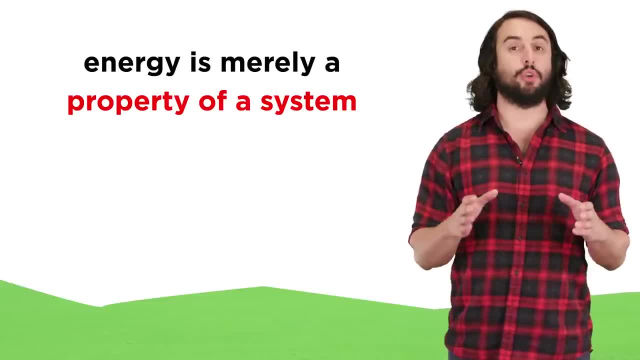 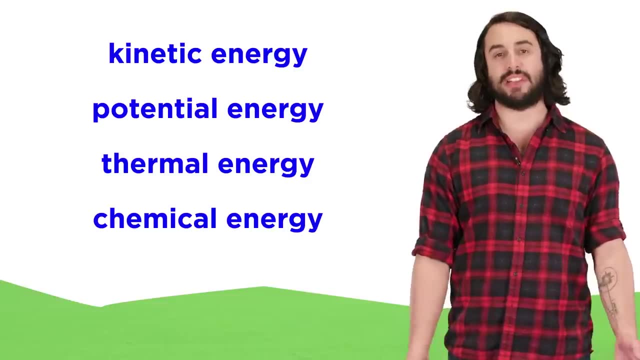 It is the property of an object or system that can be transferred into another object or system, often in the form of work. There are different kinds of energy, including kinetic and potential energies, thermal energy, chemical energy and more, and we will discuss all of these when the time comes. 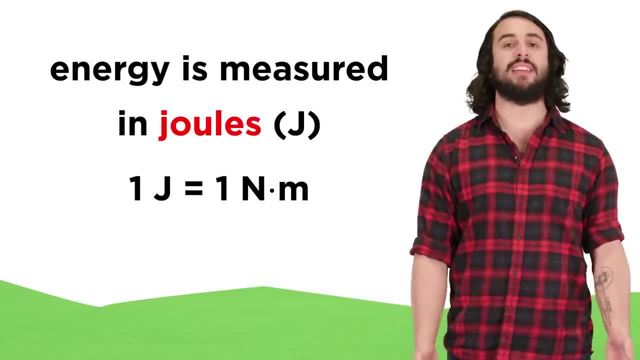 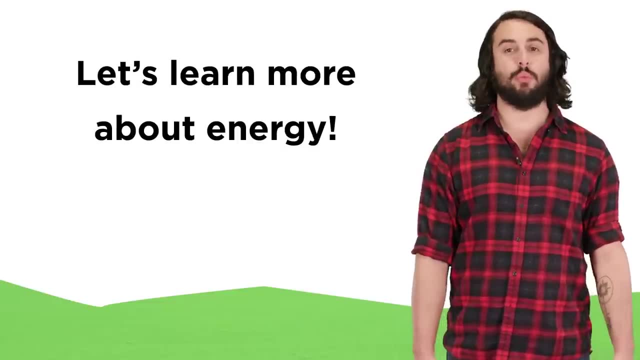 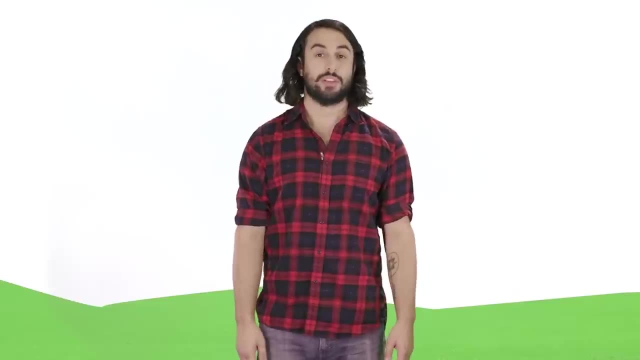 Once again, the SI unit for energy is the joule, which is defined as a newton meter, even though energy is not always transferred in the form of work. but our understanding of energy will grow as we examine it, Thank you, Thanks for watching, guys. subscribe to my channel for more tutorials. support me on. 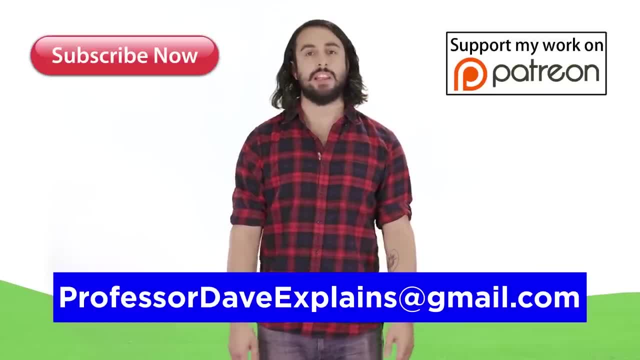 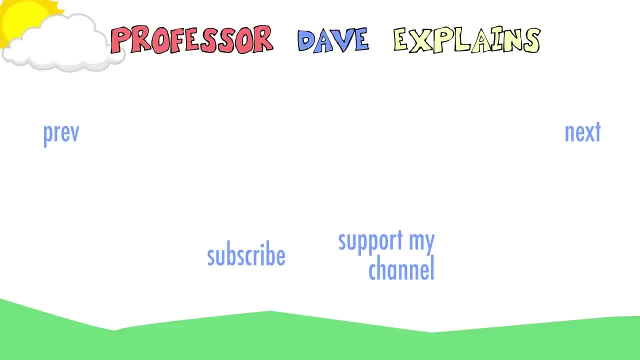 patreon, so I can keep making content. and, as always, feel free to email me, professordaveexplains at gmail dot com. I'll see you in the next one.